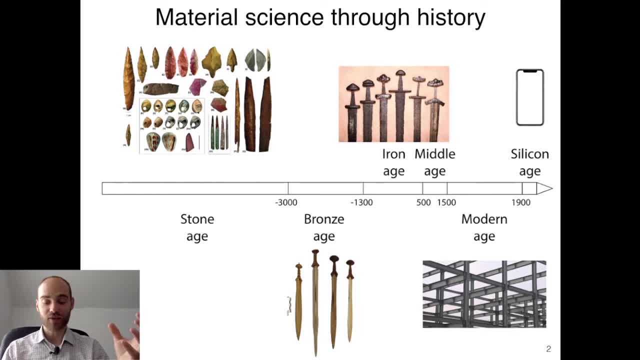 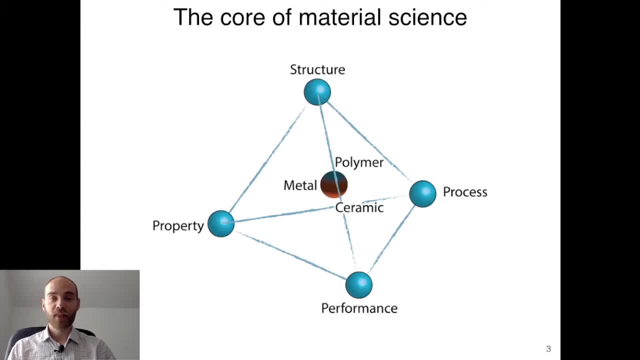 the only thing is that it's very complex, and probably one of the reasons it's a recent field is that it's actually quite complex to define. I'm assuming some of you, or at least most of you, might have chosen material because it was a mix of physics and chemistry. It's actually a bit more. 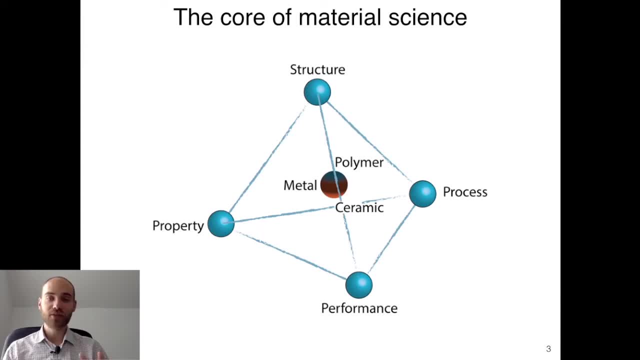 than that, and now there is more or less a consensus. let's say, in the definition, If you look at it, it's this tetrahedron. So you're probably wondering: well, what's the difference? Well, the difference is that material science is the study of the relationship between structure. 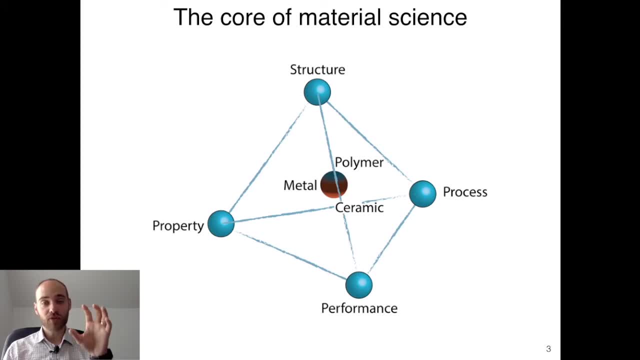 property, process and performance. So the idea is that, by using processing, we can change the structure of materials, which will influence their properties and eventually will change their performance for a specific application. And that's what we're doing: studying these relationships. 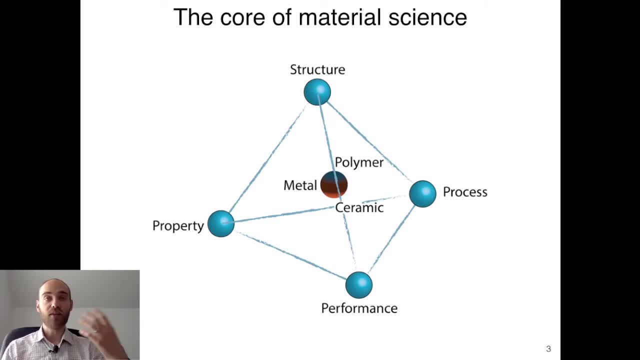 and everything is all intertwined right. So the idea is that material science is the study of the relationship between structure, property, process and performance, And that's what we're doing. And, at the core of this tetrahedron, what you can see, is that we have three different 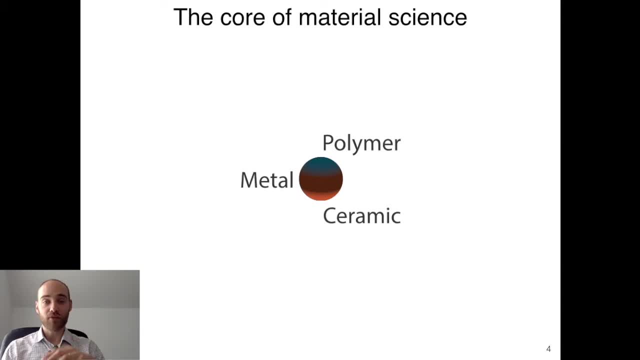 material classes: polymer, metal and ceramics. The classification comes from a very specific reason in the atomic structure of all these materials, but you will probably learn about that. But before going there, I want you to actually take a pause in this video, take a break and look around. 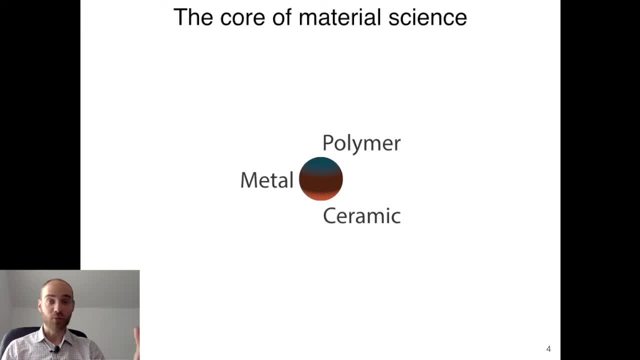 wherever you are and try to find objects that are mainly based on polymer- metal and ceramics, And what you'll find out is that you will see that these are specifically used in very different So we use metal or ceramic or polymer with very different application, and you can recognize them. 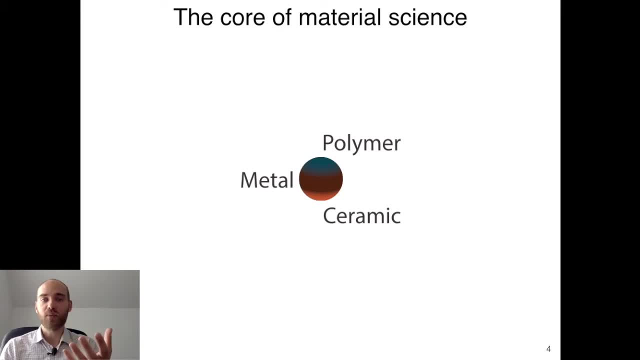 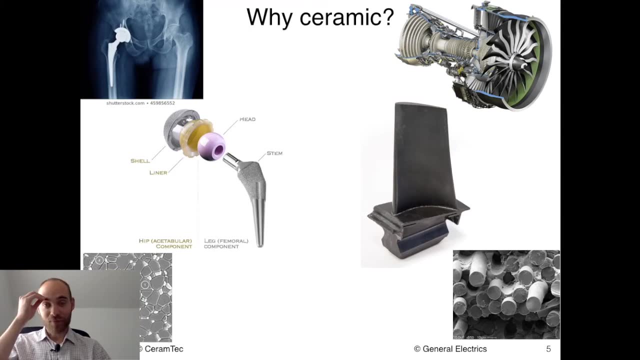 very clearly, And that's why we came up with these classes, because they are very, very different. So, after this break, which I hope you take, the next step is: I want to show you why I'm looking at ceramics, And the main thing is that, before we moved on, there's been tremendous change from the 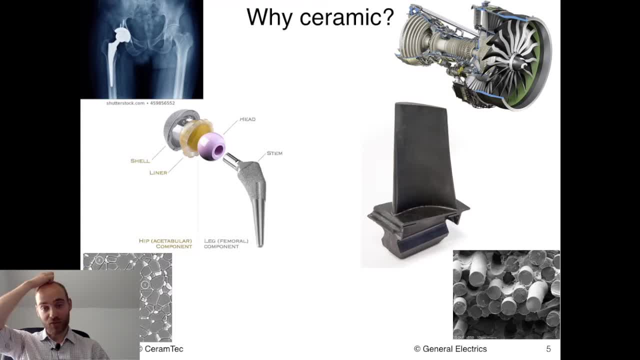 pottery that we've been using and developing in the Stone Age to the actual ceramics that we're using now, And these changes have been made on processing mainly, and on microstructure control, so that we can now use ceramic in very, very extreme conditions. 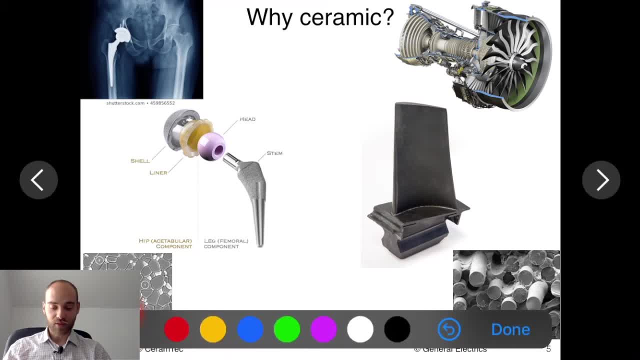 So if we look here on the slides, you will see that here we have a femoral head. so that's a part of hip replacement that is made of ceramic. And it's made of ceramic because it's extremely durable, it's wear-resistant, but it's also biocompatible, which makes it very useful. 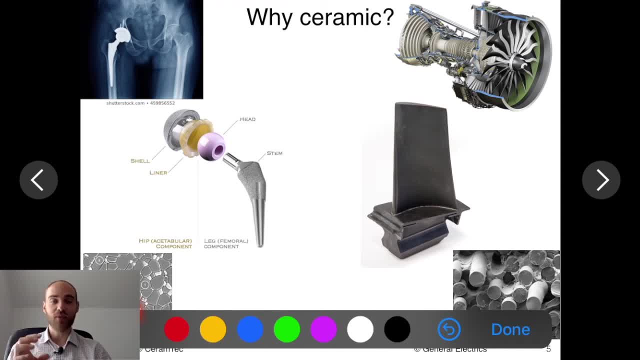 But you don't want it to be brittle, so we changed the microstructure for it to be not brittle, which is the main drawback of ceramics, so we can use them. Same story here with our, with now. I mean, it's a very recent development. now some turbine engine blades are 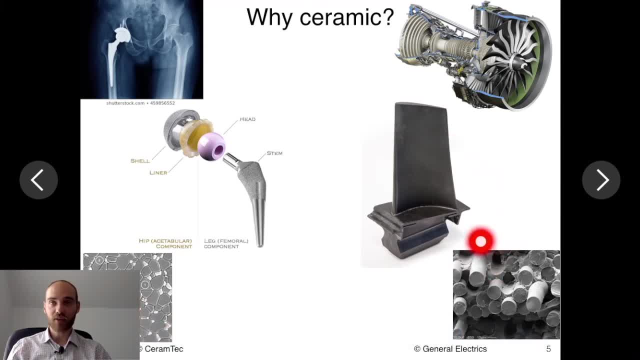 made of ceramic And again we changed the microstructure here and you can see you have very long fibers here to make the structure very tough, so very resistant to cracks, so that we can use the natural heat resistance of ceramics to use them in turbine engine where if we increase the temperature of an engine, 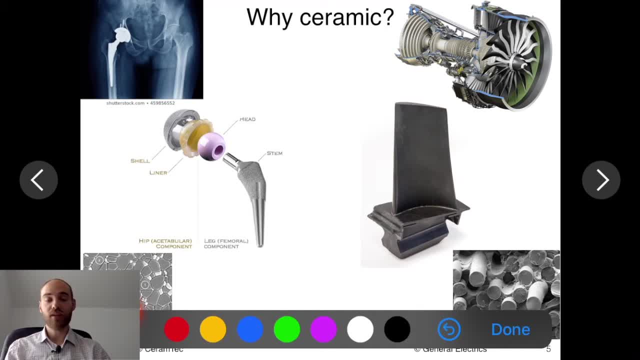 it will actually be more efficient. So we use the natural assets of the ceramics- biocompatible or heat resistant- and by changing the microstructure we've been able to remove or actually temper some of the main drawbacks, which is their brittleness. 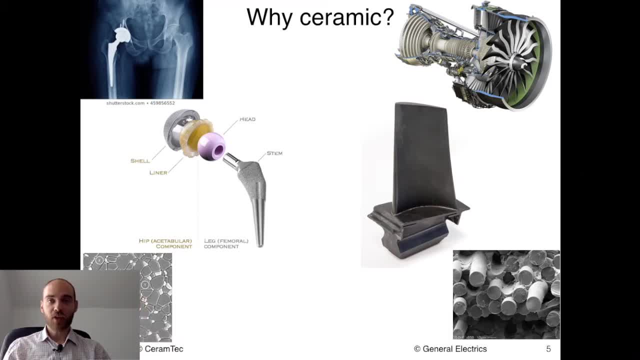 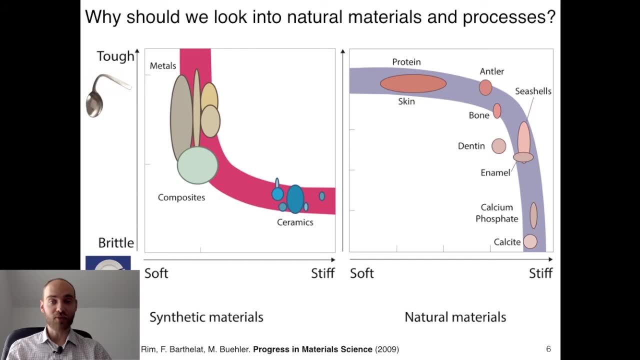 so we can use them in this specific application. So that's what has been going on in research and I'm going to show you actually another type of way to reinforce ceramic which found its way in natural materials, and that's the research field I'm working on. 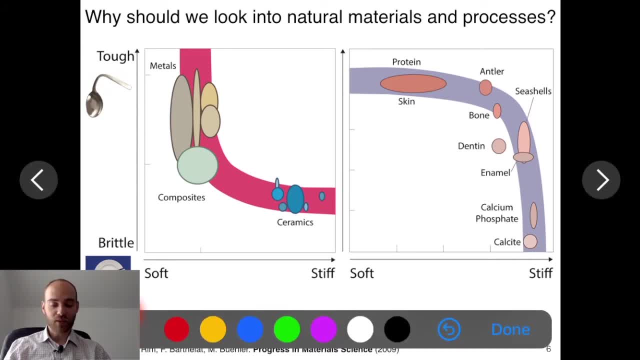 And if you look at here on these slides, what you'll see is that if we go from, if we plot synthetic materials from brittle here to tough, so we find you know ceramics very brittle, so very low. metals very tough, very high, and we have composites here. 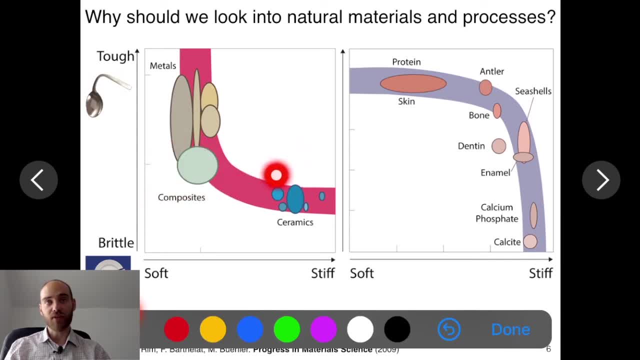 and from soft to stiff. so we have ceramics that are the stiffest and metals. here What you can see is that if we plot, if we put composites or if we mix these two things, we usually end up with what is called a banana curve right, And we end up with the. 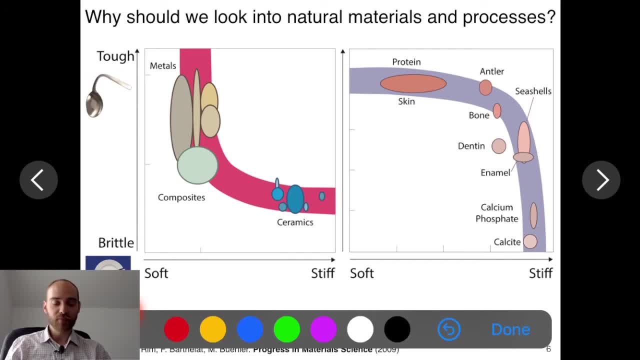 somehow a combination of these properties, but not a great one, right? And the thing is, if we do the same thing with a little trick, with natural materials, and you can see that we have here, we have some protein or the skin, so these are extremely tough but very soft and these are. 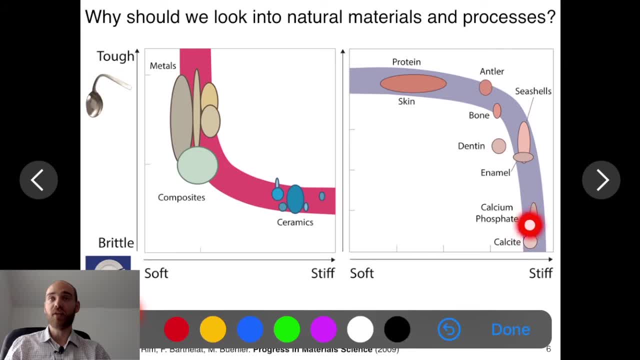 the mineral that most of natural materials are based on, so calcium phosphate or calcium carbonate, but also very, very brittle. Well, what you can see is that if we, when nature's- you know when the natural materials are made- what you can see is that when you mix these two, well, 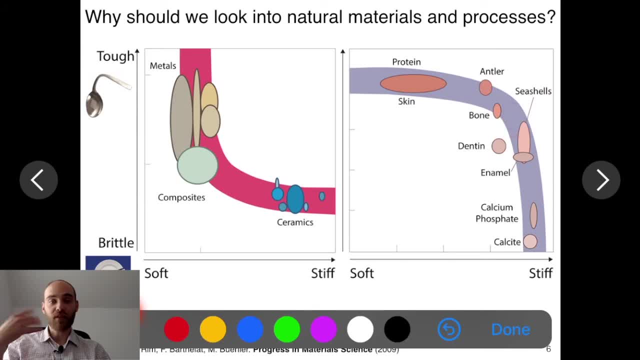 you end up here this time, so you actually get the best of both. You have something that is extremely stiff but also extremely tough, And there is nothing. you know the we know the composition we are able to make each individual materials of these, these natural composites. 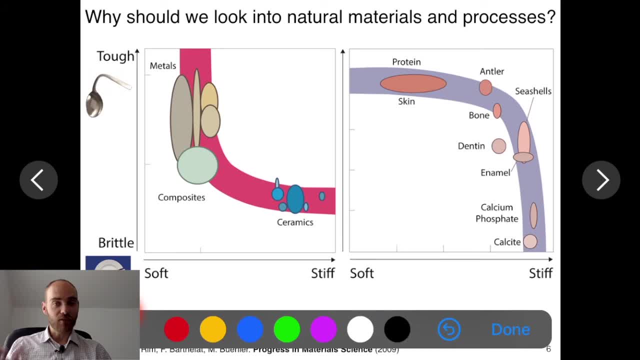 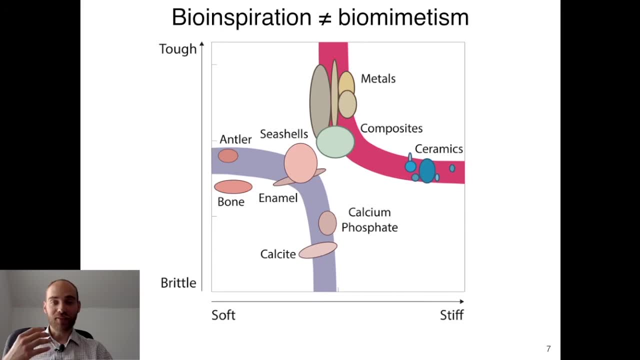 and nothing. you know. it's just in the microstructure, in the way they are they are arranged, that there is something very interesting. So now I don't want to try to, you know, convince you that we should make sea, we should make airplanes out of seashells, right? 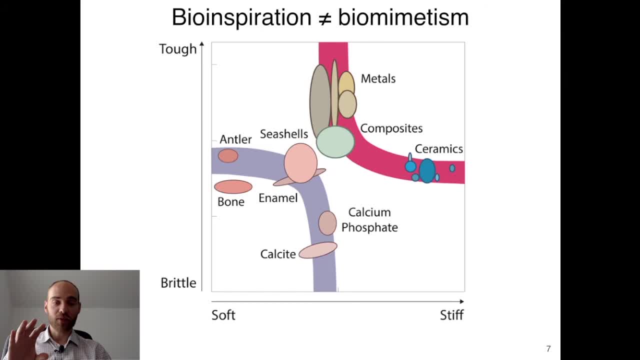 If we actually plot them in the same graph, you would see that most natural materials are worse than any synthetic material. So our idea is not to try to reproduce one-to-one seashells or bone or other material, but what we're going to try to do is understand where you come from. 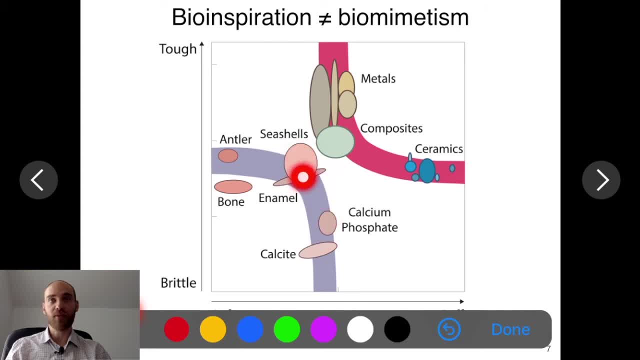 how you go from this material, this base material, to these composites, So that if we use that for ceramics, it means we can basically end up up here So having something that is extremely, extremely stiff, extremely strong, but also extremely tough. 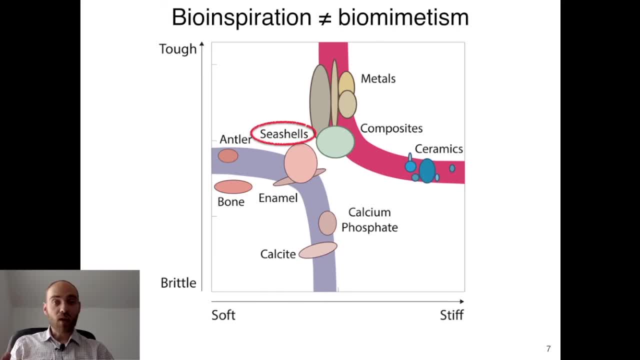 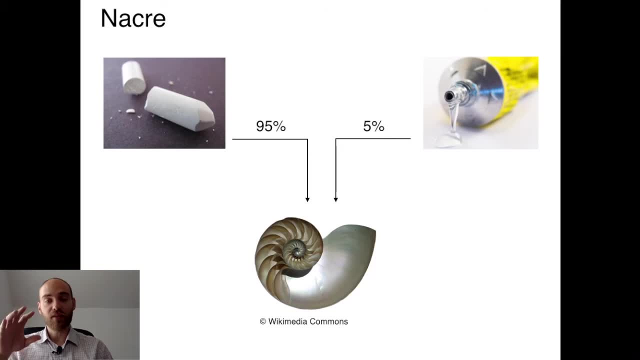 And so we're going to look at the example of seashell because we want to understand why this improvement, where this improvement occurs. look at the specific example of seashell. and it's made of these main constituents called nacre or nacre, and if you look at the composition, it is 95 percent chalk, calcium carbonate. 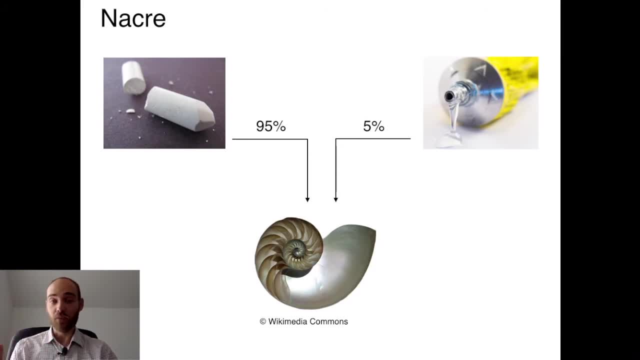 and five percent of a protein. that is basically just a glue, um, just like any glue that you can find, a synthetic one. however, when you, because of the way these two components are arranged at a very fine scale, you will have an extremely tough materials and- and i know, it might be very 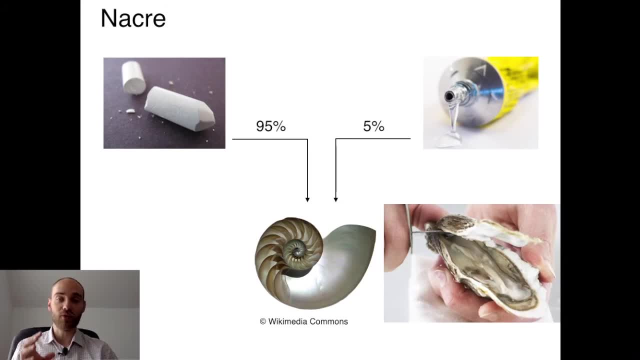 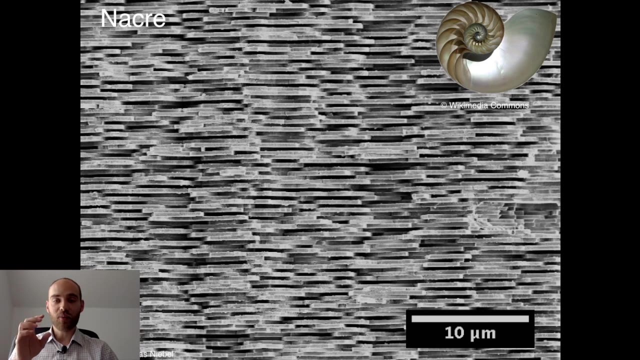 a very french problem, but if you ever try to open an oyster, you will realize how tough it is to actually um and how dangerous it is to actually open this, these seashells, and they are the again made of chalk and glue. one of the reason and the thing i want to really briefly show you is that 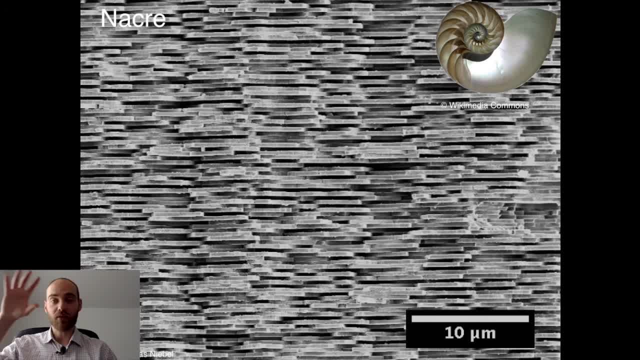 it comes from the microstructure. so it's the way these materials are arranged in space, and you can see they are made of tiny platelets, very tiny, so 10 micron in size, arranged perfectly, stacked together with just a fine layer of glue in between, and so that's it's. 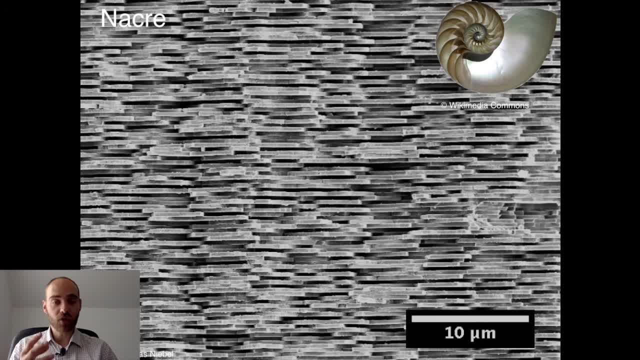 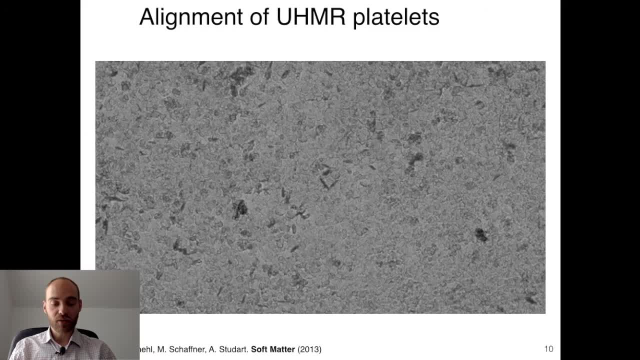 called brick and mortar architectures, and this structure is able to dissipate a lot of energy instead of just failing in a brittle way. so my research has been trying to to figure out a way to mimic this structure with actual synthetic ceramics- not with calcium carbonate, but something a lot stronger: the 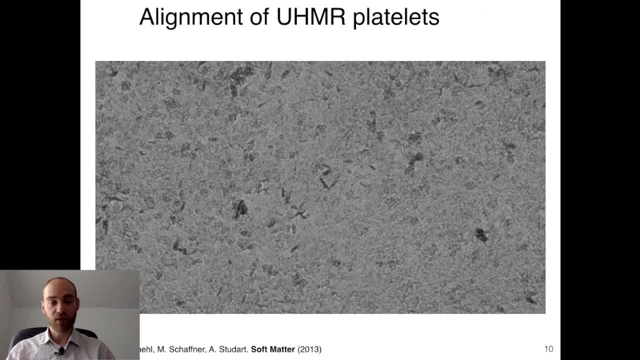 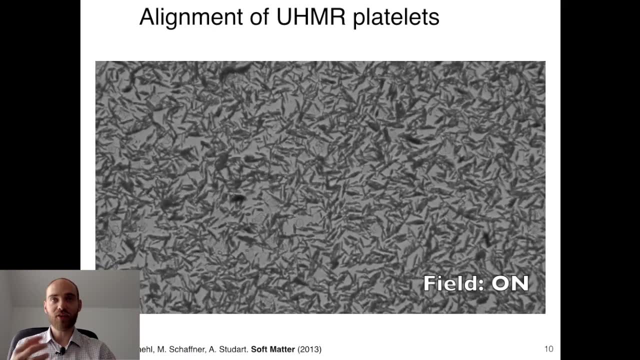 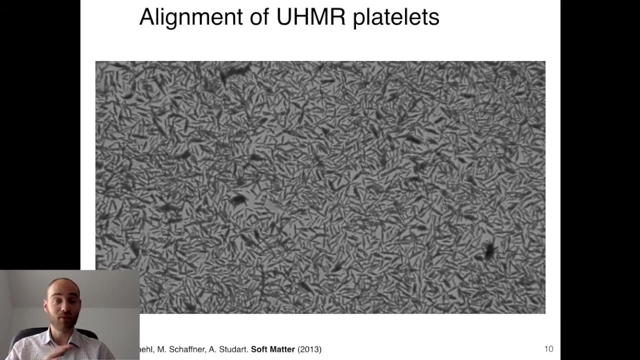 things that we can put in hip, but trying to mimic this, the same structure, and try to see if it makes it better. so one way we can actually start controlling and and making these things. we can't use the same process as nature does. it's just too slow. even if we could, which we can't, it's just 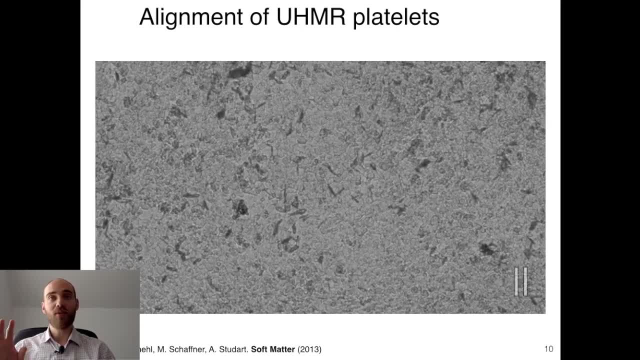 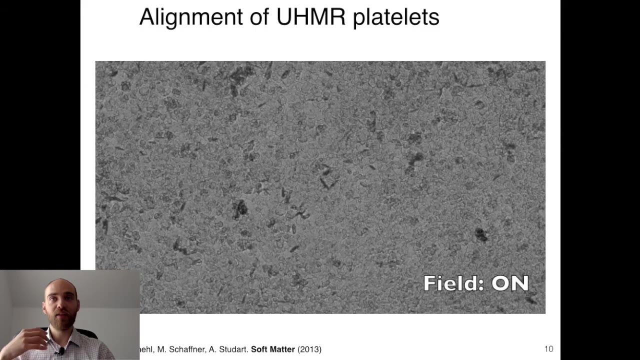 impossibly slow. so one way we use we do is actually trying to take these individual platelets and control the orientation one way or another. and what you just seen in the video and if i just go back and play it again, what you see is that when we put a small magnetic field- and we're talking a fridge magnet now- and these 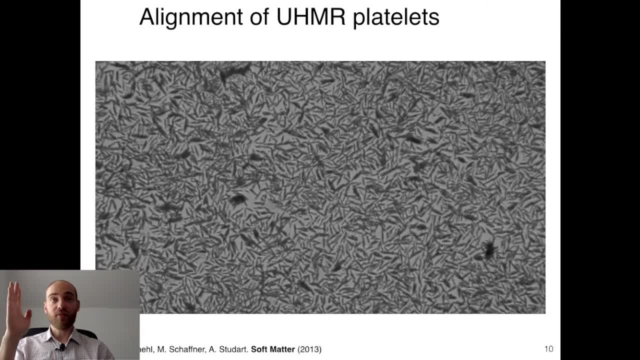 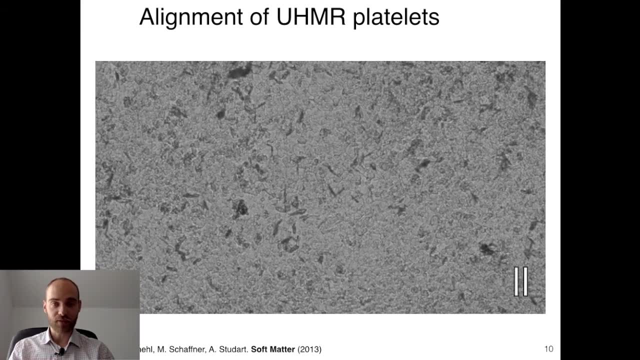 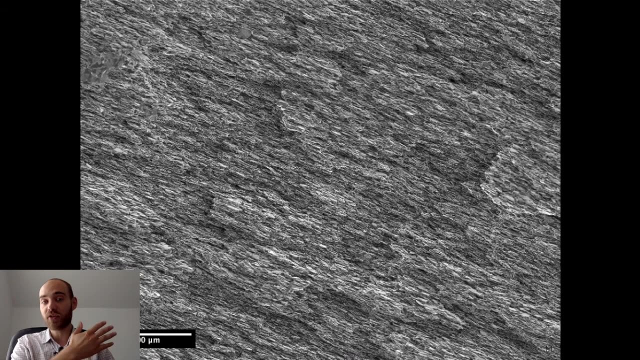 are platelets of of sapphire. you actually you are able to control the orientation very quickly and very nicely, so this allowed you this process to up in at eth in switzerland allowed you to mimic this microstructure very well and if you remember the the picture i showed you before, you can see that they they very much look the same. 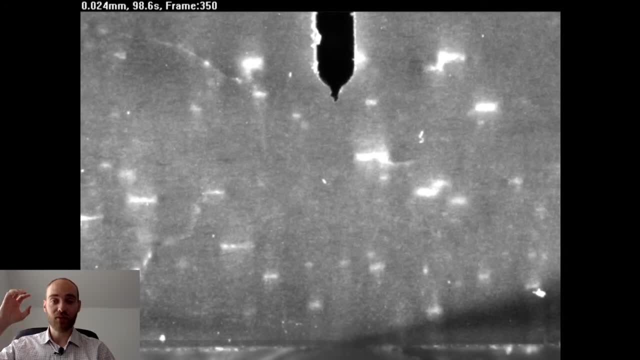 i can't go into that much detail. but if you take this sample and if you heat it and if you make the just the right um fine tuning of the interface between each of these individual aligned platelets that we've seen before, while you end up with a ceramic so purely, 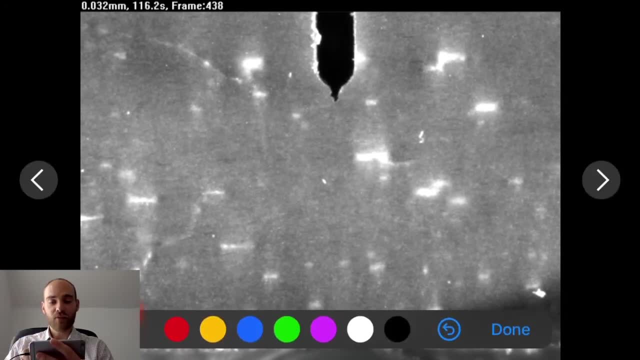 a ceramic that behaves like this. if you can see, if you look here, you can see a crack developing here, but that grows in a very, very steady fashion. you even have another crack growing here in a very steady fashion. so by mimicking the, the structure of naker, we've been able to make very tough ceramic. 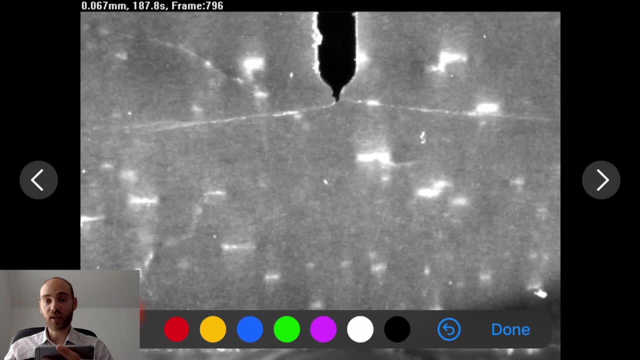 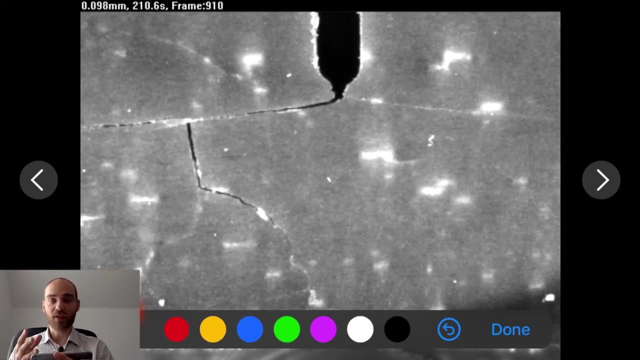 as well, where the crack, instead of just you know, breaking the sample, exploding the sample, it's just growing in a very stable way, which gives you actually some time. it's it's basically a warning if you would use these parts in application. so warnings say, okay, we need to change this piece. 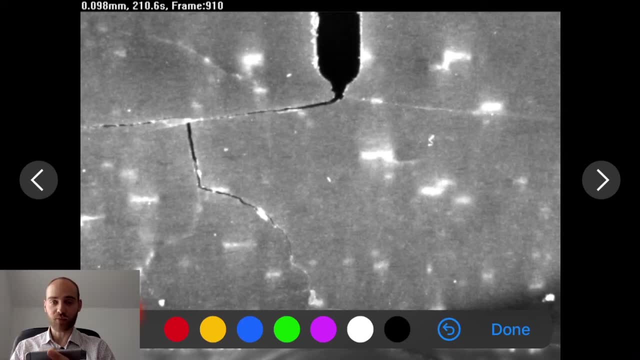 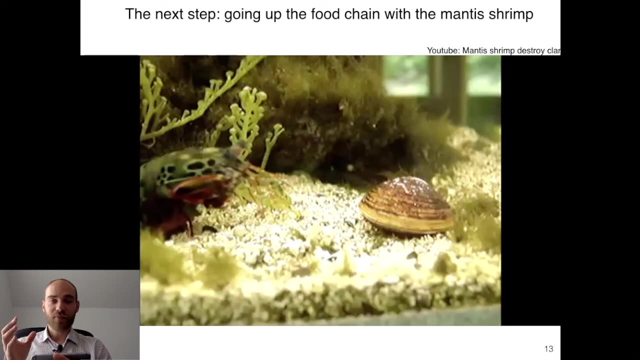 but it's not going to just explode, and that's what you want for structural application, right? finally, um is for the, the follow-up. so now we've been able to make this material, the follow-up is: uh, there's an easy way to to do a follow-up, let's say for us is that we can. 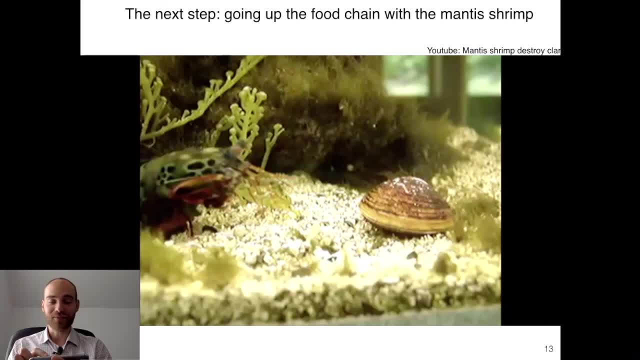 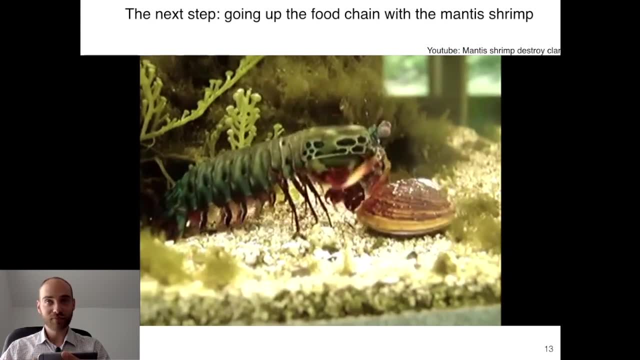 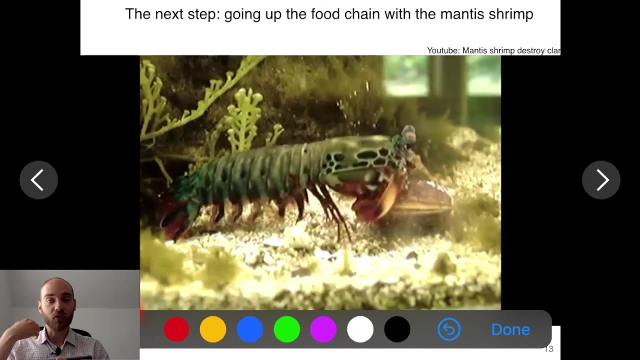 actually go up the food chain. um, and i just want to show you again a small video, and this is, uh, it's called the mantis shrimp and you can see it has a tiny, it actually has a tiny hammer here that is using to, you know, just smash makers. so the seashell, the stuff that we've been